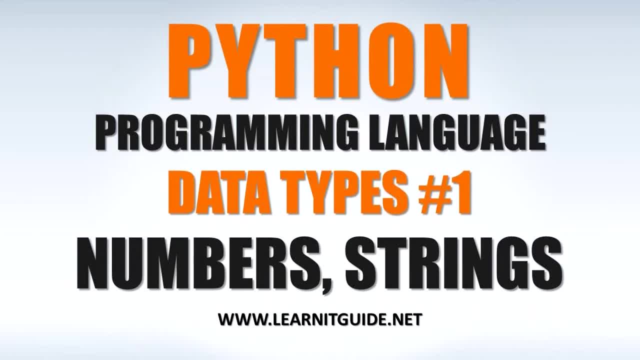 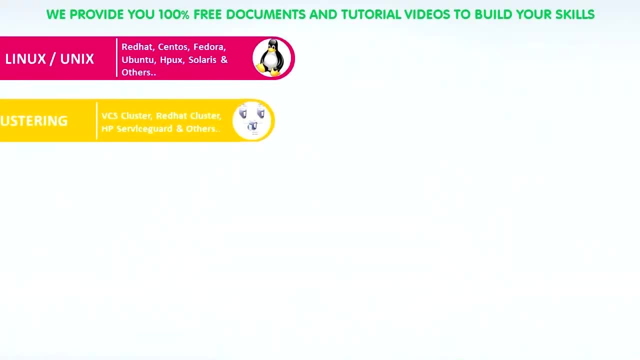 please leave your comments in the comment section and subscribe our YouTube channel for more updates. And you are watching LearnIT Guide tutorials. We provide you 100% free documents And tutorial videos to build your skills. For more updates, stay connected with us on. 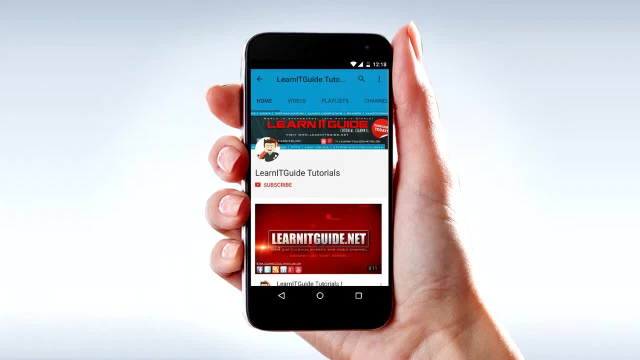 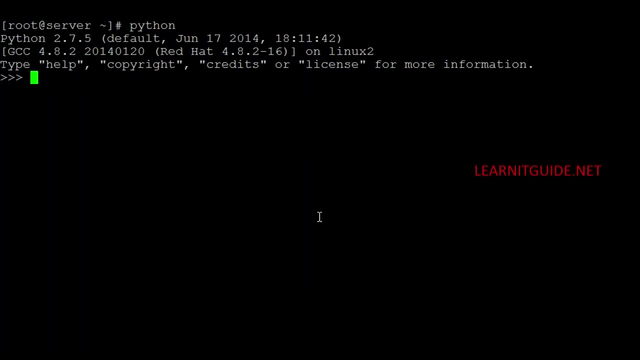 social networking sites and subscribe our YouTube channel. Go to youtubecom and search for LearnIT guide tutorials. Hit subscribe button to not miss any updates. Click nearby bell icon to get notification immediately. Let's move on to data types. Data types are nothing, The type of the data you are storing in the memory for the variables, For example. 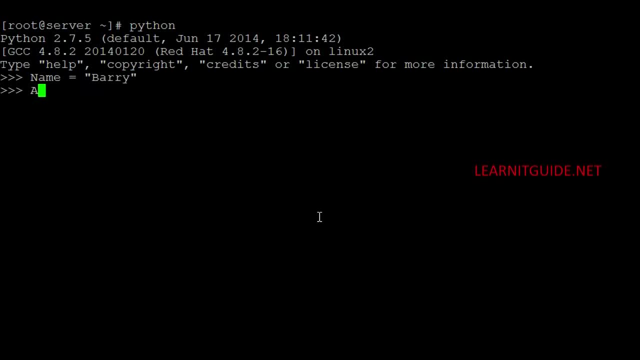 name equal to Barry, age equal to 30.. So these are the two variables: name and age. For name, the value of name is Barry and the value of age is 30. Here one is in alphabetic characters and we call: 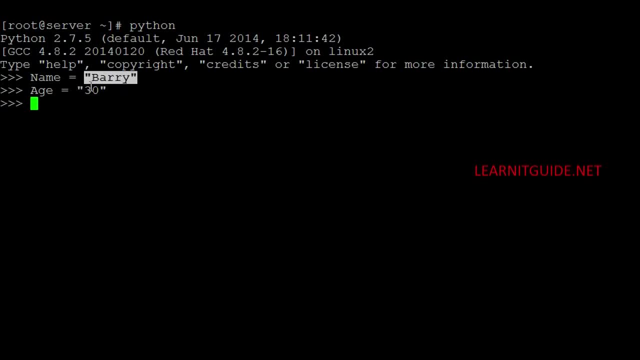 that as a strings and the age is in numbers format. So this is what the data types in Python. So Barry is in strings and age is in numbers. So Python has five standard types: Numbers- I just write over here numbers, strings, list, tuple and dictionary. So these are. 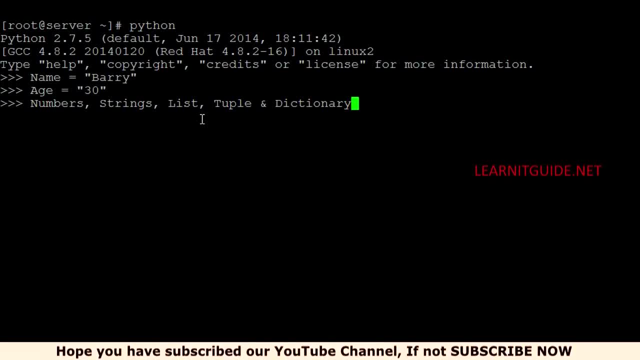 the five standard data types we have in Python. Let's see each one of these One by one with examples. So let's start with numbers. Python numbers is a data types of Python and the data you store for a variable would be in the number types. So this is a data type of numbers. 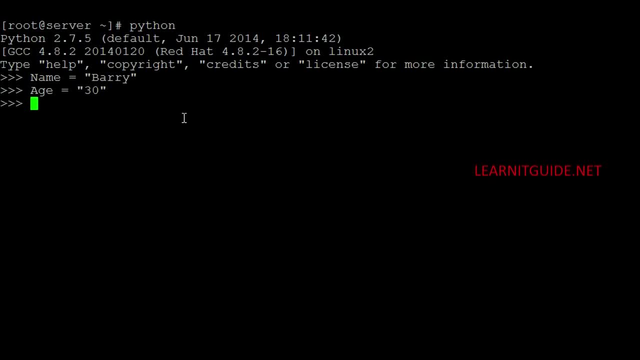 So we call this as numbers, data types. For example, apples equal to 20 and grapes equal to 10.. So I have two variables: apples and the value of apples is 20 in number format, and for the grapes I have set the value 10.. 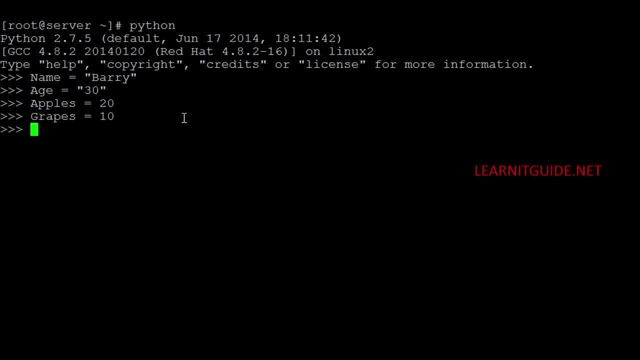 So both are numbers data types Here. so number data types may have some of the types, not only complete integers. for example, not only. it would be 20.. Sometime the value of apples or grapes, whatever. sometime the variables value would be something like 10 or it might be floating point: 10.0, 11.5, 11.4. these are floating points. 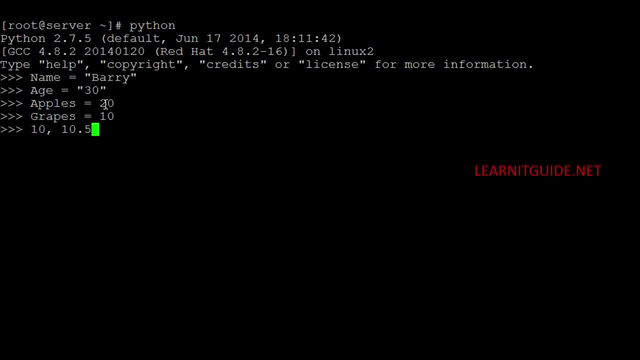 So we cannot say that the value would be only the integer numbers. It might be integers or it might be floatings as well as it might be long numbers. Again, you may have complex numbers, Something like 5., 5., 5.. 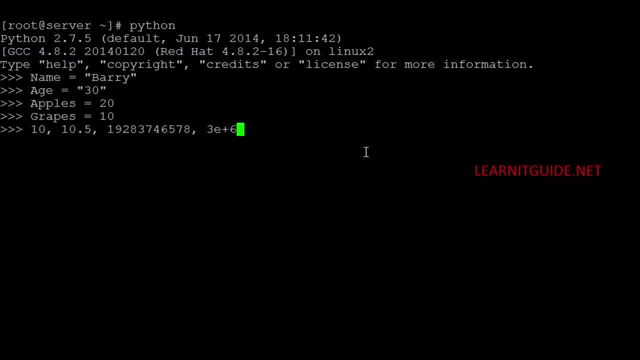 5. 5. Like this. So these are complex numbers. So, with respect to numbers, data types, you can have these types of numbers: Integers, long numbers, floating numbers and complex numbers- Alright. So, along with numbers, we can use some operators to perform mathematic functions, like additions. 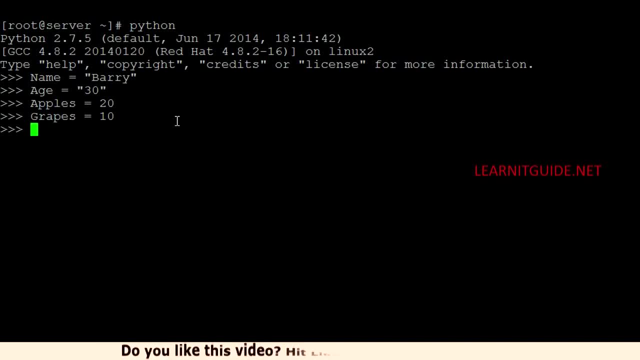 subtractions, multiplications, divisions and other modular functions, For example, if you wanted to add these two to know your number of stocks in your departmental stores. So what I do? total equal to apples plus grapes. I just called the variable to know the value of it. 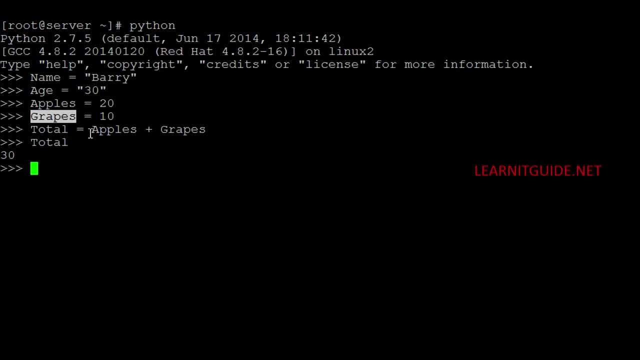 So addition of these two is 30. Even if you give, like this, 30. And you can do multiplications Using this operator. So these are operators equal to: is operator, plus is for addition operator and hyphen or minus for subtractions. 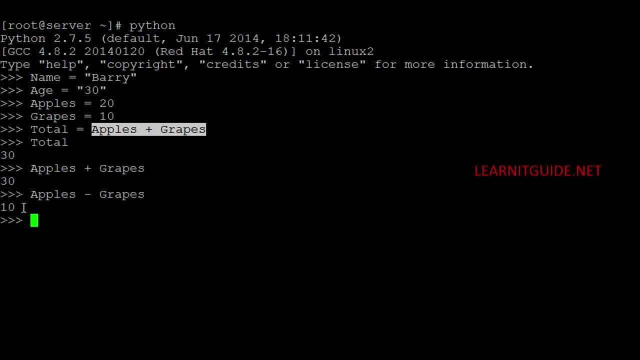 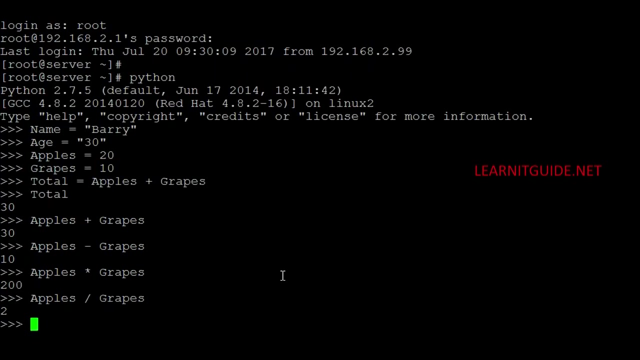 So the value of these two, 20 minus 10, is equal to 10.. And you can do multiplications and you can do divisions. So these are the basic operators. normally we do for the mathematic functions As well. as you can have more number of mathematic operators, you can use that as well. 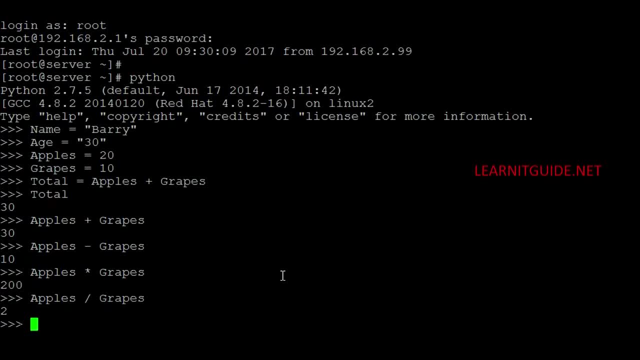 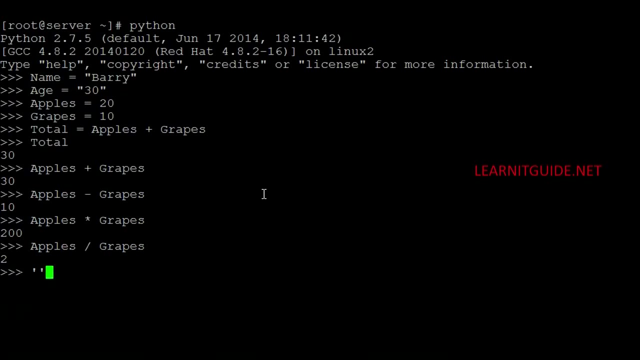 And I will explain you more about operators in the upcoming session. we have a brief session for that: operators. So so got an idea. what is number, data types and how to use it. Let's move on to strings. So strings are nothing but characters are enclosed within single quote or double quote. 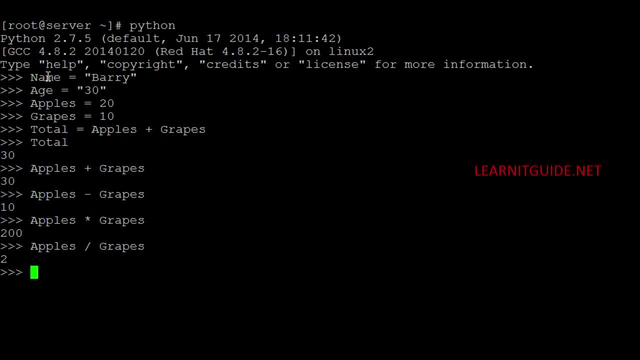 Even in this example You can have a look. This is my variable and the operator and the value of it enclosed within double quote and this is considered as a strings. The value, whatever you are giving within single quote or double quotes will be considered as a strings. 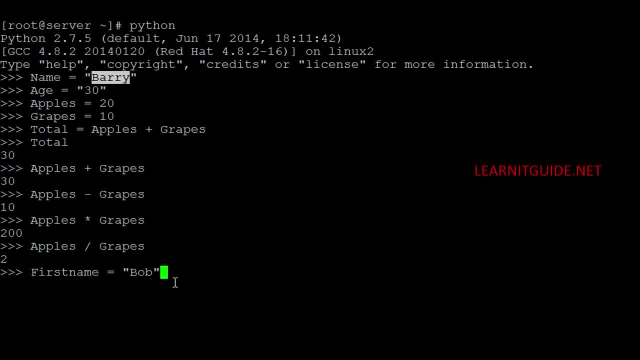 For example, this is strings. These are also one more strings: first name and last name. So these are strings, data types. here We can match these two with operators as well, Not only along with numbers, even with strings. you can match the value of these two. 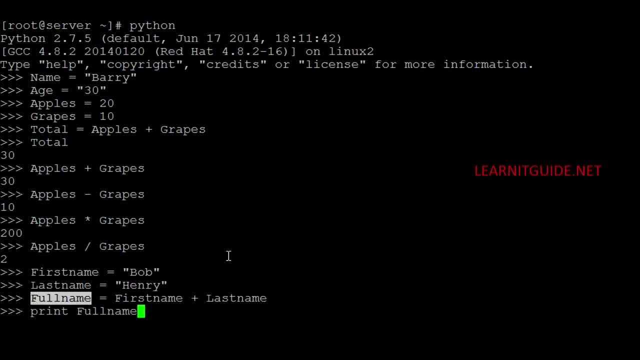 So called the print function, to know the value of full name. now Bob Henry Here. What you have is you don't have a space in between these two values. If you want to leave a space, what you have to do instead of printing directly, just double. 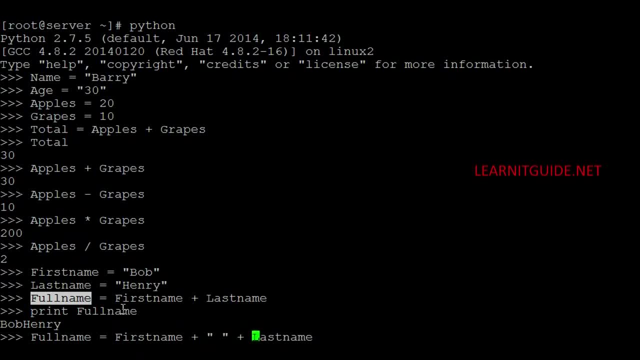 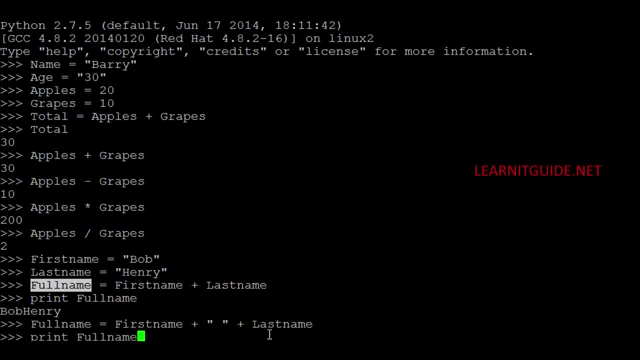 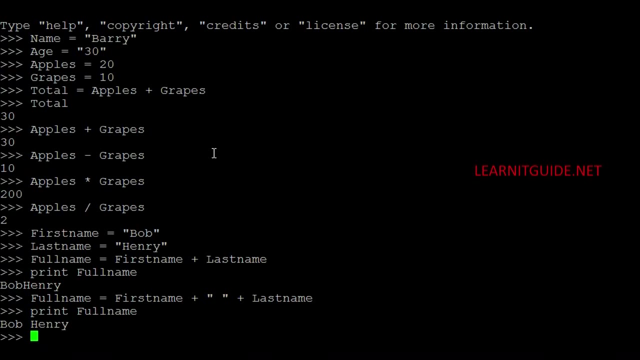 quotes, space again plus first name, then space, then last name. Let's see the output Now you have a space in between first name and last name, Bob Henry. Here We have one options to get the substrings of strings. 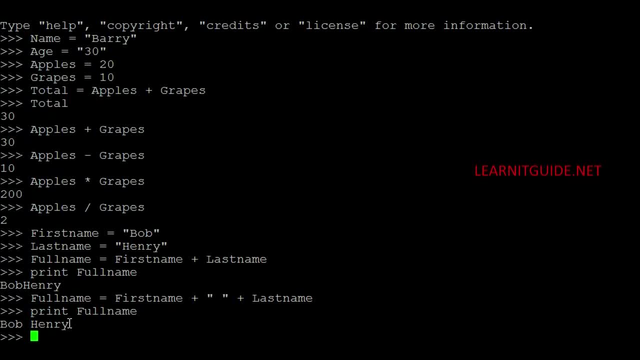 For example, this is a strings and if I call substring some of these characters, not the complete strings, some of the characters from the strings. So that is what substrings of a strings. So to get some value of a strings you can use slice operators. 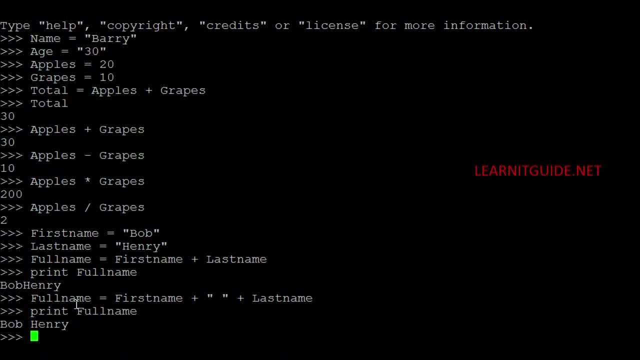 Let me show you an example. So If you wanted to only print Henry, or if you wanted to only print Bob from here, then you can use the slice operators with the square brackets. So let me show you that: print full name within square bracket. 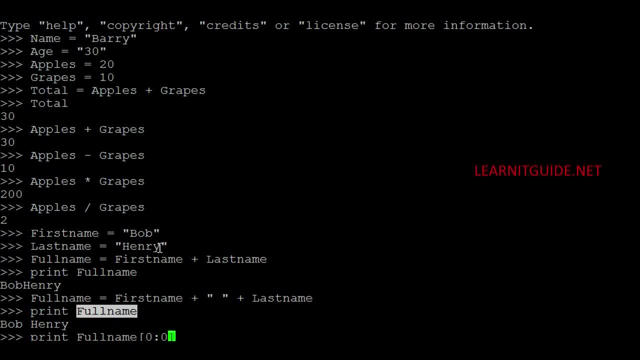 You have a syntax something like this: Okay, So what does it mean? Normally, The machine language, The internet, The syntax of these strings will start with zero. zero, then 1,, 2,, 3,, 4,, 5,, 6,, 7,, 8.. 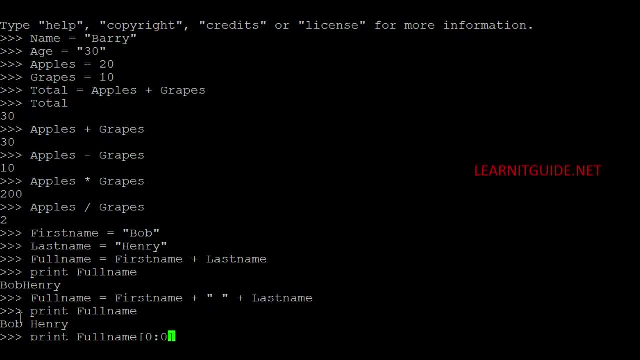 It starts with zero For the machine language. if it is a human, how do we read normally will not start with zero. We start with 1, 1,, 2,, 3,, like that. So this is to start with. you have to use the machine language: 0,, 1,, 2,, like this: 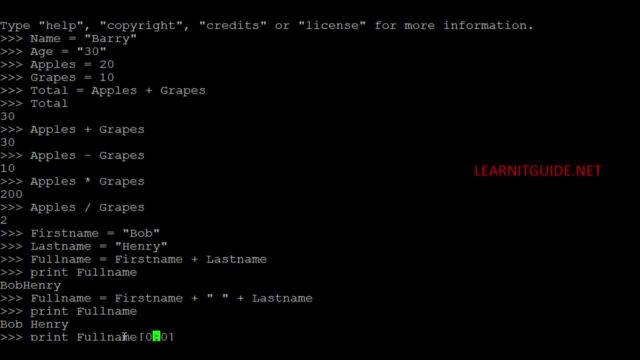 And by default The first position would be zero And for the end position you have to use in the human format, For example, if you want to display from the zero position to third digit, 1,, 2,, 3,, because 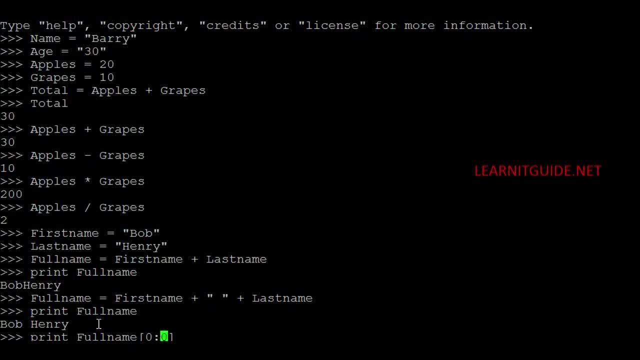 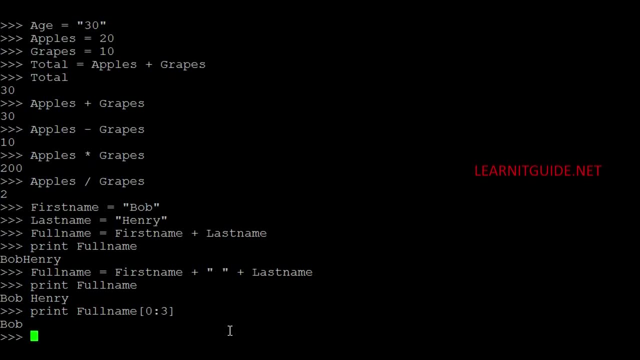 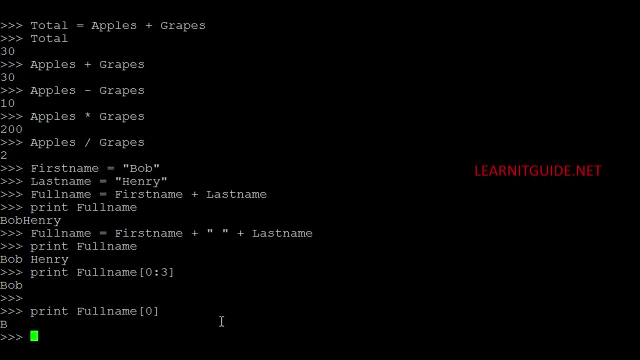 I'm going to give the end position, So I will be giving in the human format. So 1,, 2,, 3.. So I just give instead of zero. I just give three. Bob, Now if you want to print from the first position, then just give, like this: 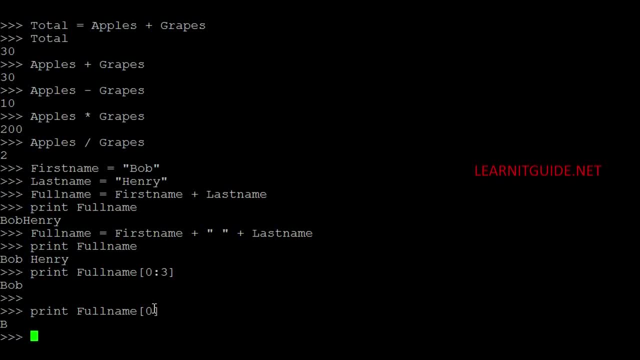 So it will print only the particular number. And if you want to print till something, seven, So you got from the zero position till the end. So the end is in human format. You have to give 1, 2,, 3,, 4,, 5,, 6,, 7..